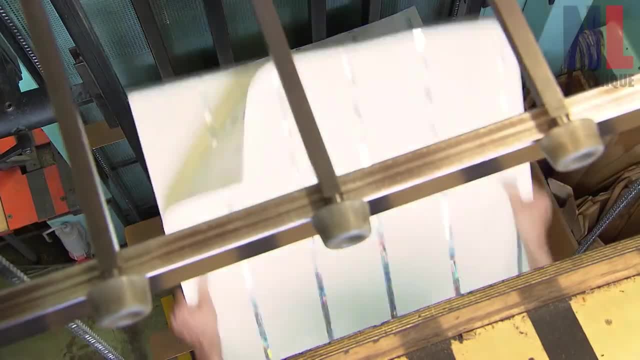 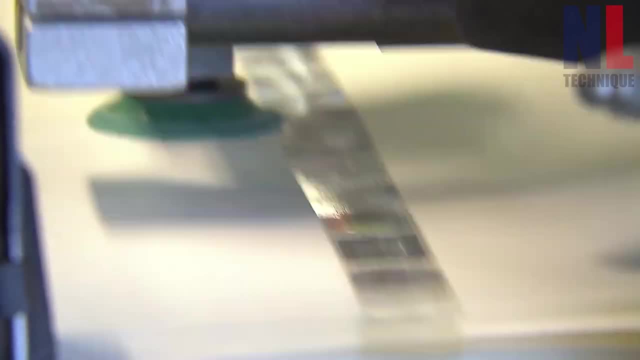 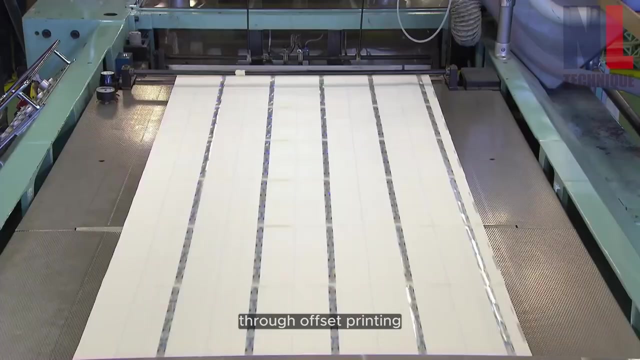 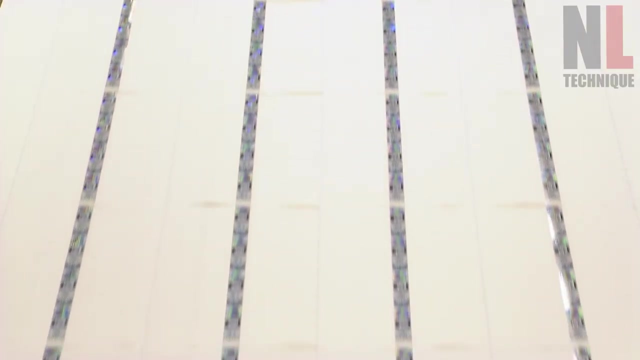 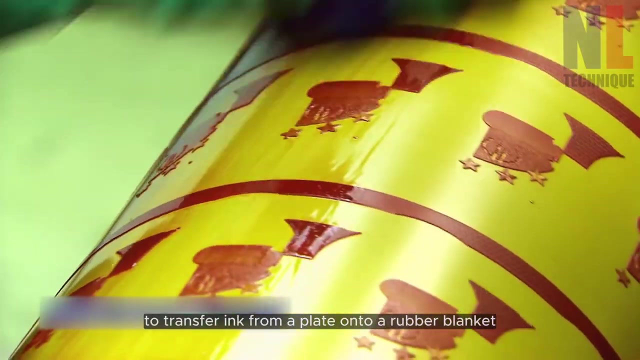 Once the paper is ready, it's time for the banknote designs to come to life through offset printing. Offset printing implies that the paper is ready to be printed. The banknote employs advanced technology to transfer ink from a plate onto a rubber blanket, which then transfers the ink onto the banknote paper. 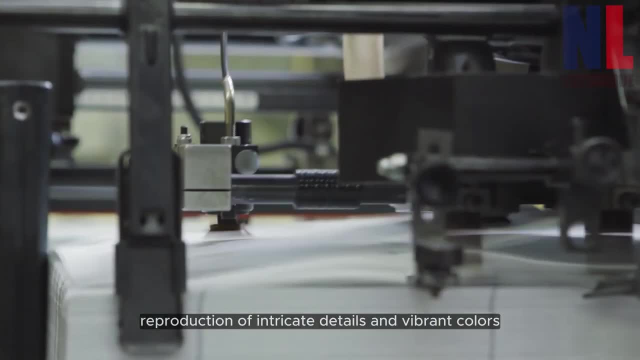 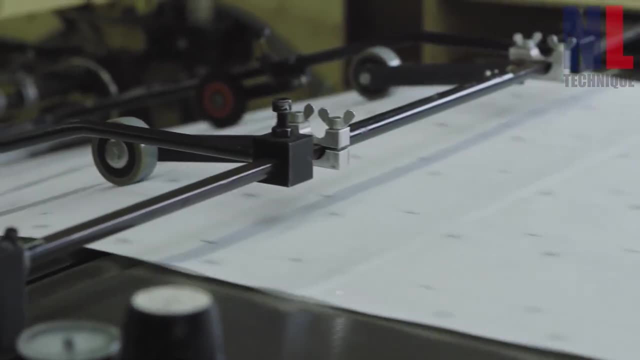 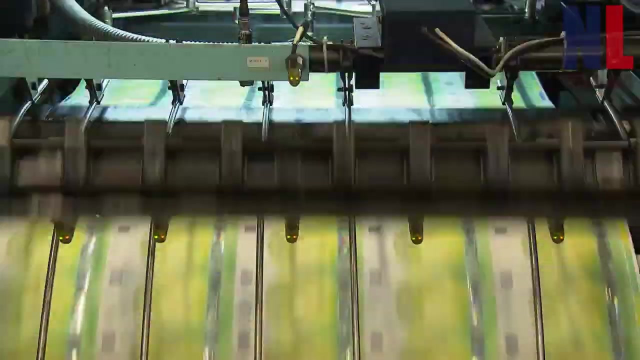 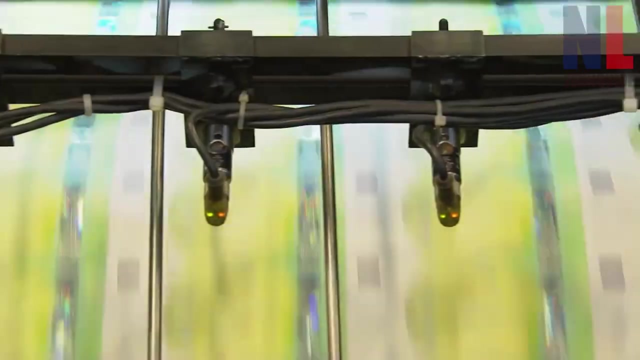 This process ensures high quality and accurate reproduction of intricate details and vibrant colors. For example, the paper ink can be printed in the form of a card and printed on a string, a paper cloth or a cloth, and then printed into a simple represents a piece of paper. 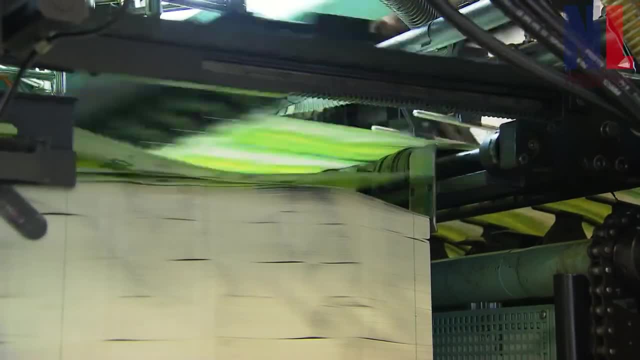 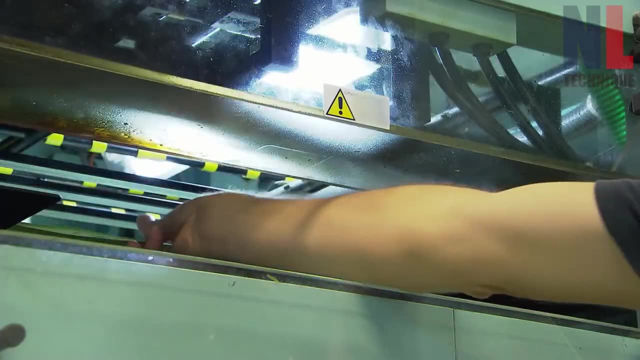 The paper underneath is used for the printing of the paper. The criss-cross nossos are made from a thick, clean paper that is laminated and then glued together into a thin mix of ink and paper. This is where we begin the making of the banknote and the cut. 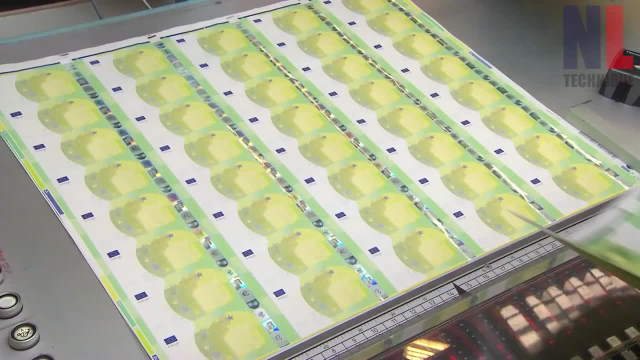 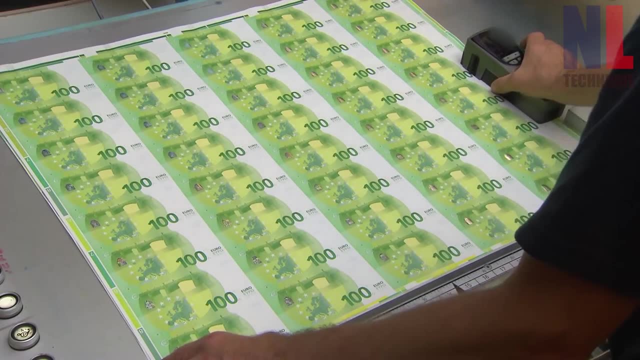 We start by creating an outline of the banknote, a cross-section that is used for the pattern. The very first step for the print is to cut the paper pieces in half. This is done by hand. I start with two pieces of paper: one made from performa and one from a copper plate. 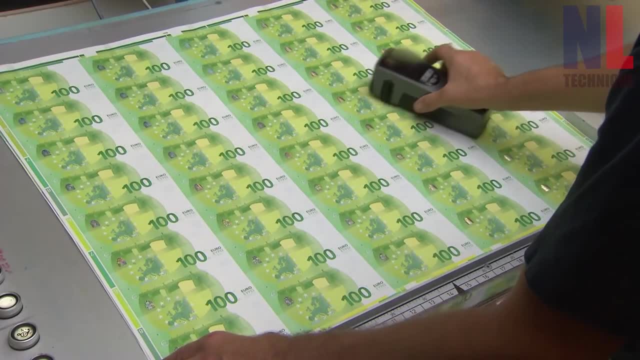 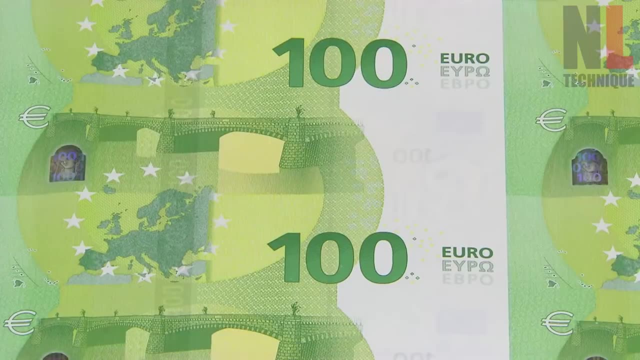 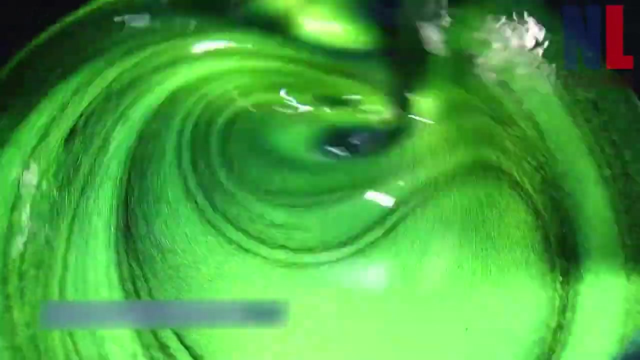 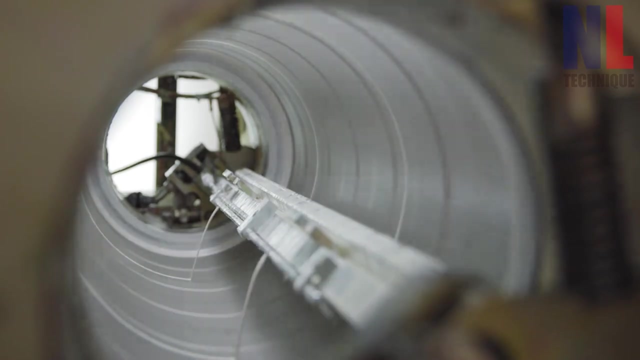 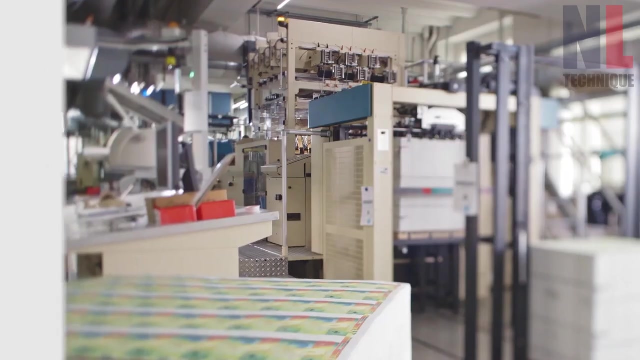 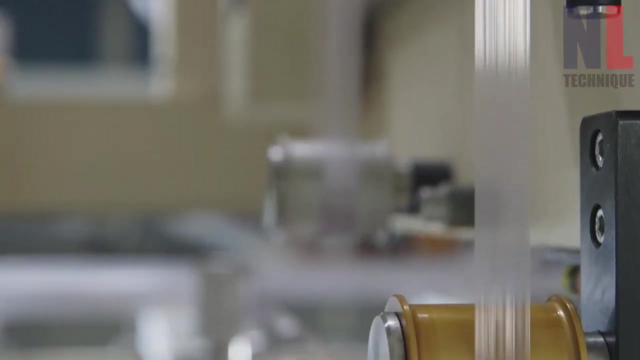 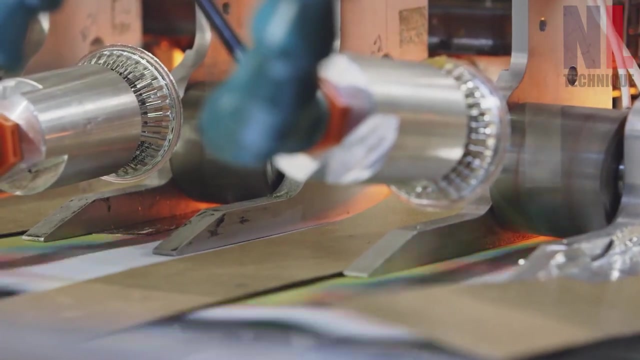 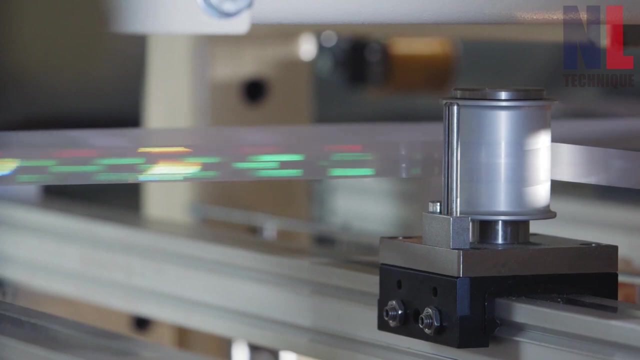 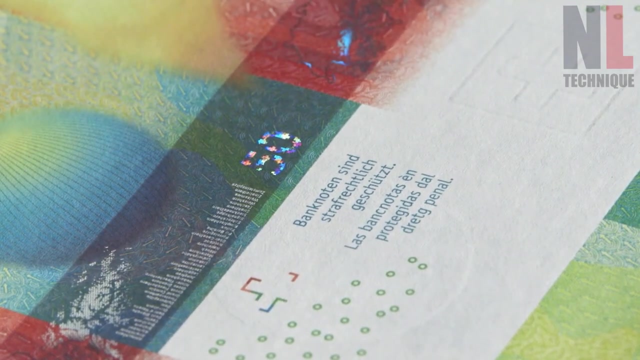 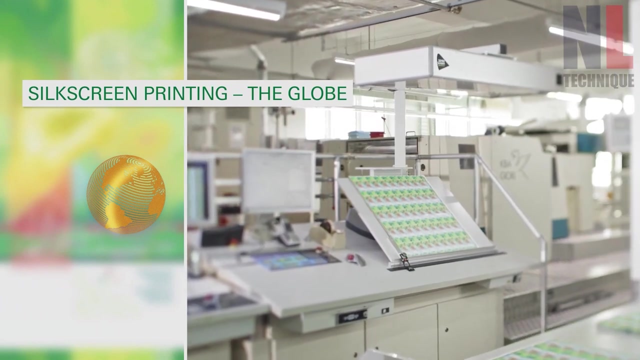 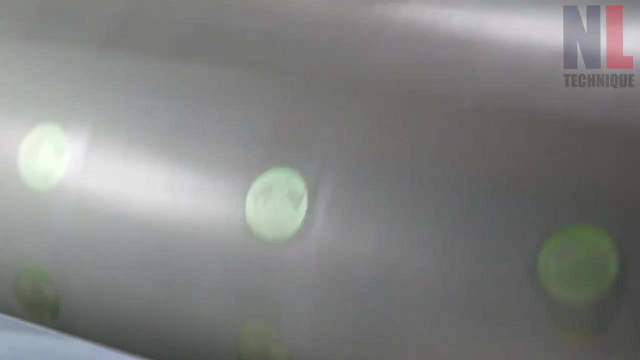 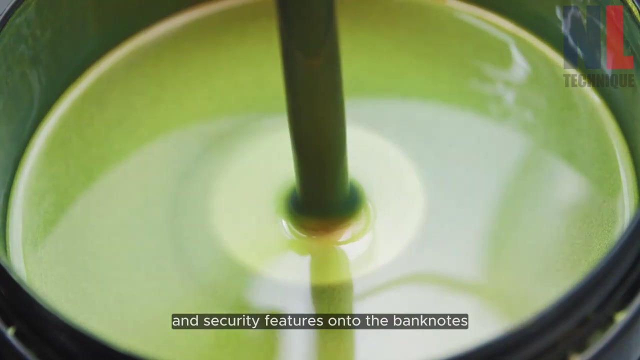 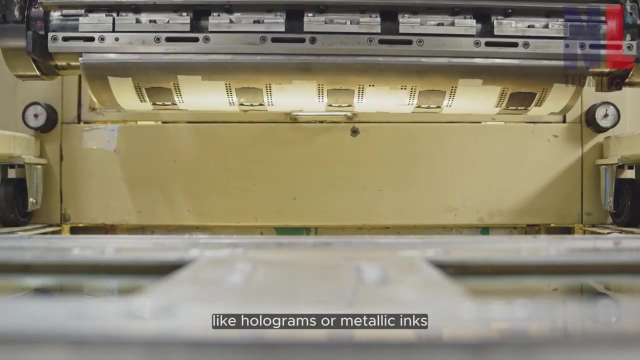 I cut the paper into thin strips. Next we have silk screen printing, also known as screen printing. Thank you for watching. Thank you for watching. This method allows for precise placement of unique elements like holograms or metallic inks, enhancing the security and aesthetics of the banknotes. 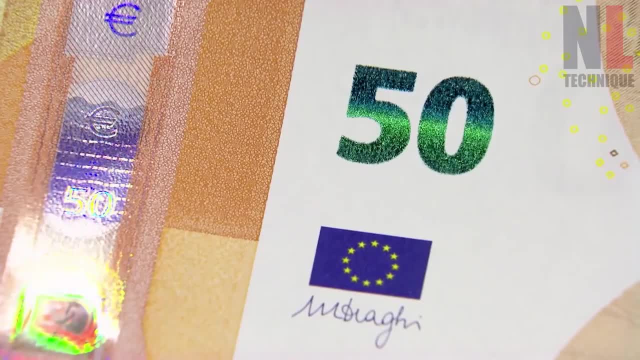 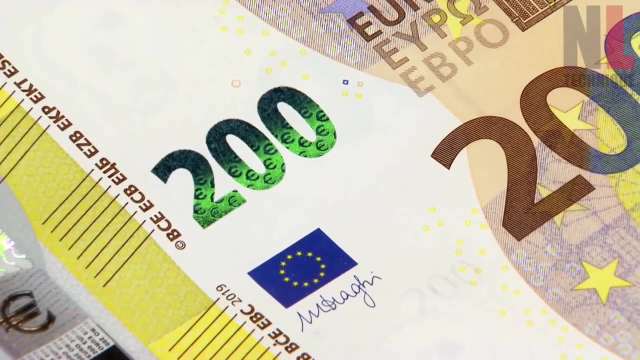 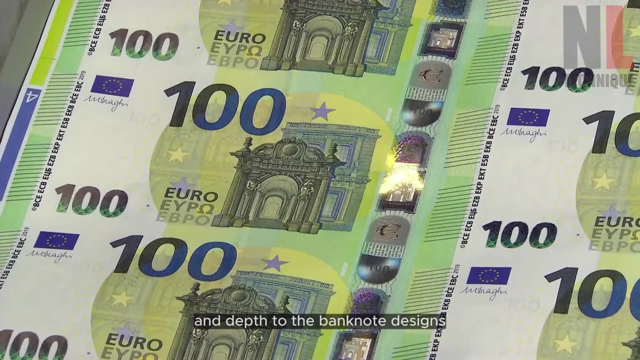 This method allows for precise placement of unique elements like holograms or metallic inks, enhancing the security and aesthetics of the banknotes. Now let's move on to intaglio printing, a process that adds texture and depth to the banknote designs. 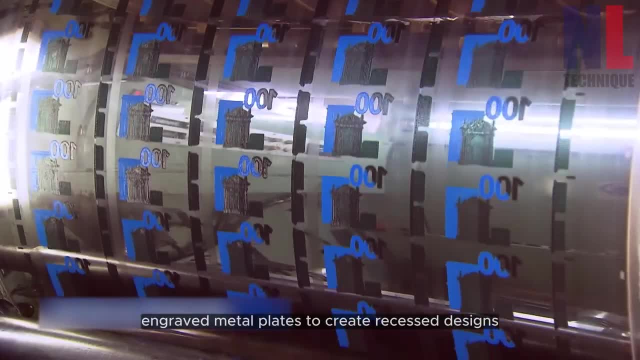 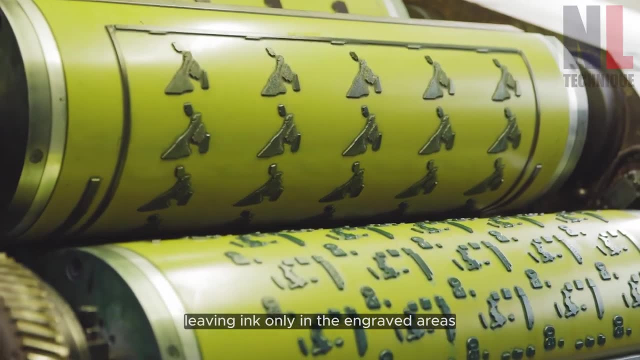 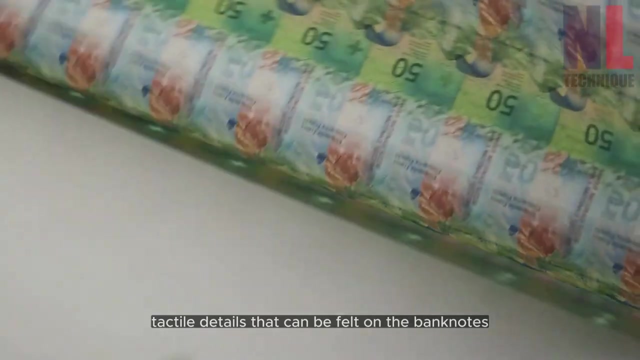 Intaglio printing utilizes engraved metal plates to create recessed designs. Ink is applied to the plates and excess ink is wiped away, leaving ink only in the engraved metal plates. The paper is then pressed against the plates, resulting in raised tactile details that can be felt on the banknotes. 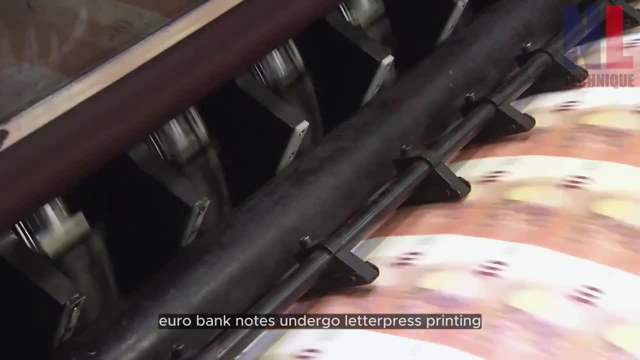 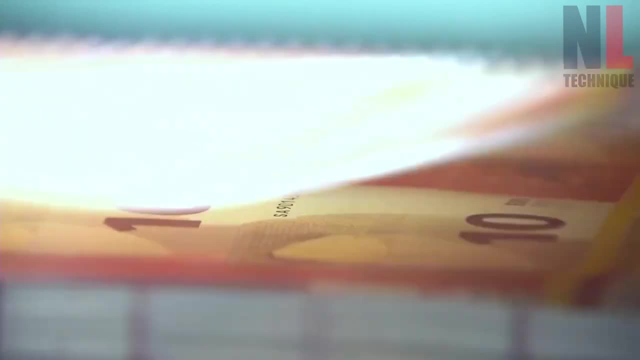 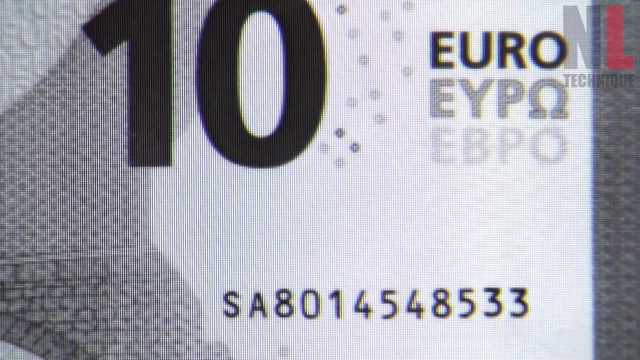 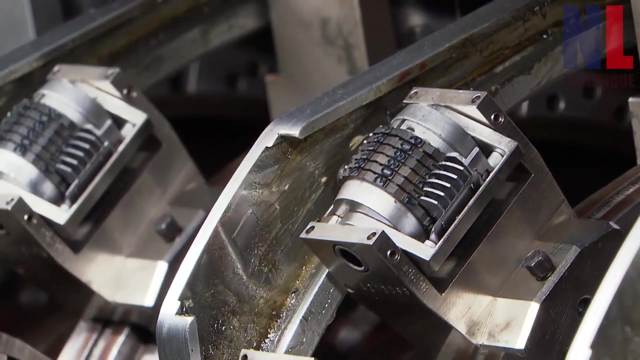 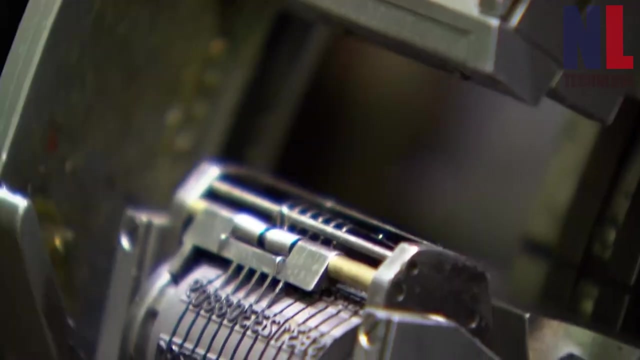 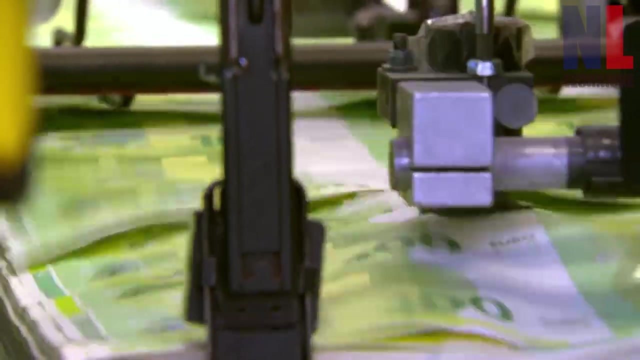 In addition to intaglio printing, euro banknotes, undergo letterpress printing to add additional security features. In addition to intaglio printing euro banknotes, undergo letterpress printing to add additional security features. In addition to intaglio printing euro banknotes, undergo letterpress printing to add additional security features. 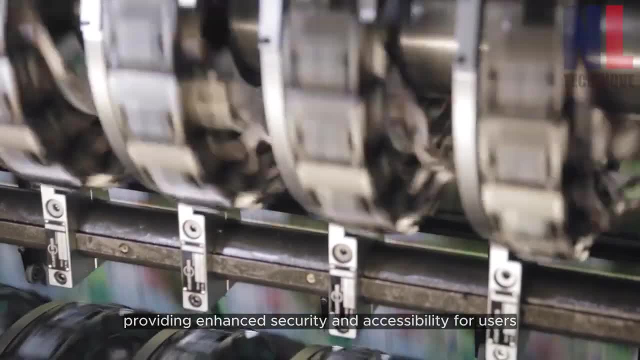 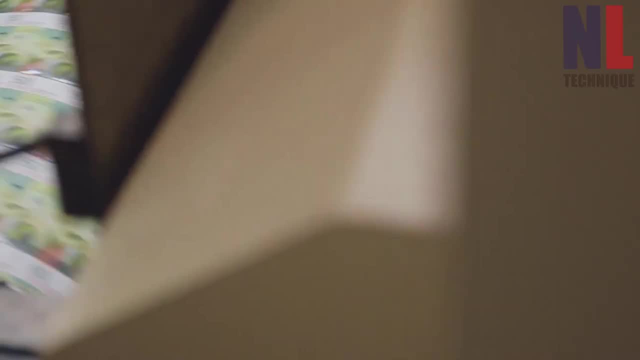 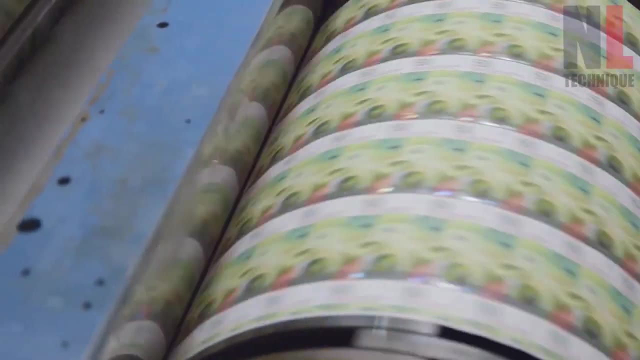 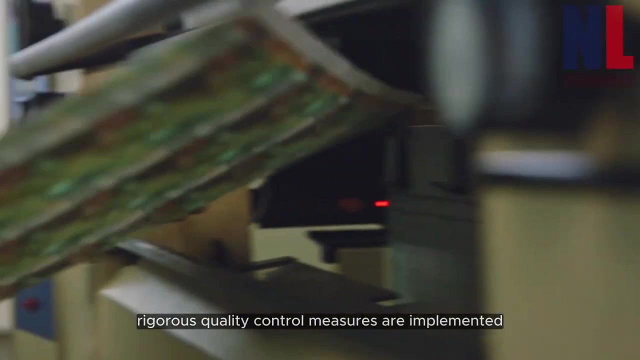 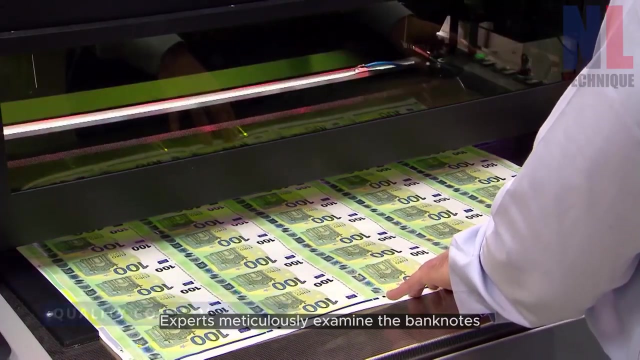 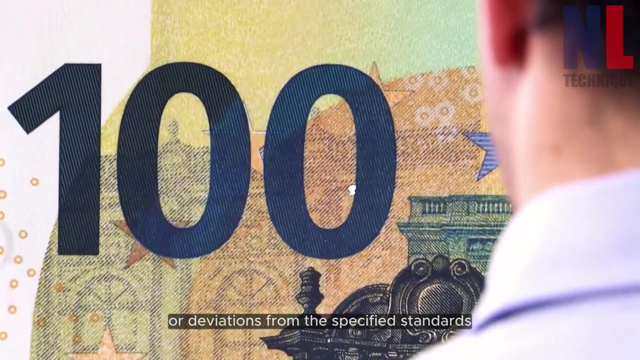 patterns or Braille markings, providing enhanced security and accessibility for users. throughout the production process, rigorous quality control measures are implemented to ensure the banknotes meet the highest standards. experts meticulously examine the banknotes, checking for any flaws, imperfections or deviations from the specified standards. this meticulous 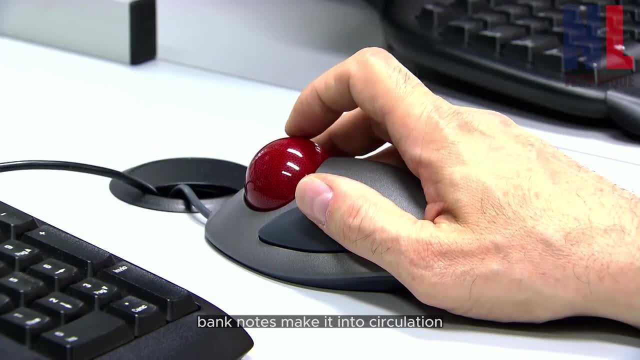 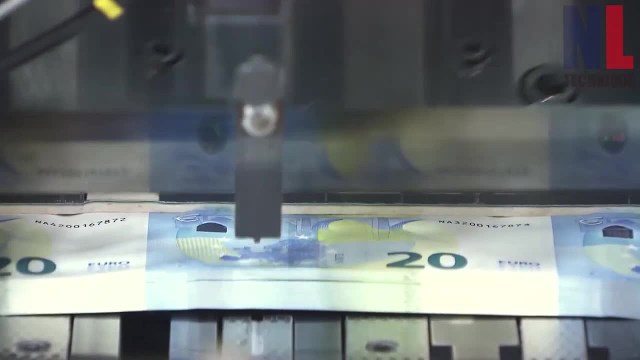 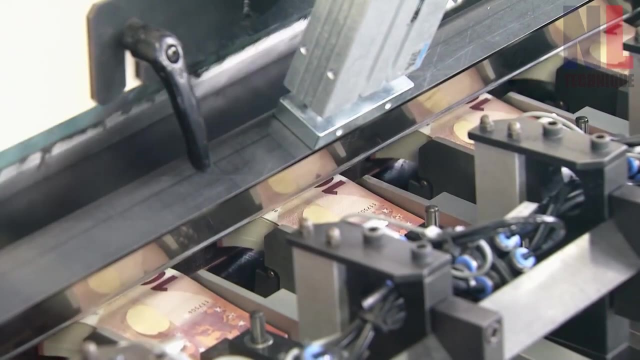 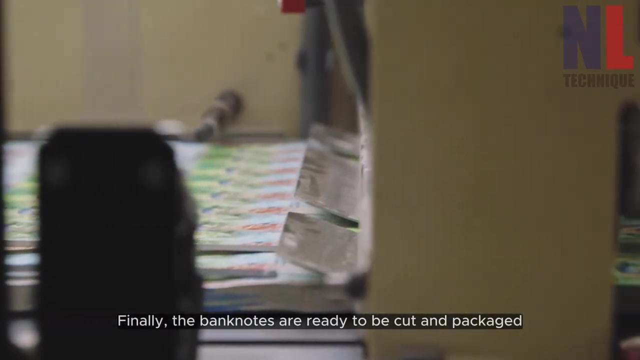 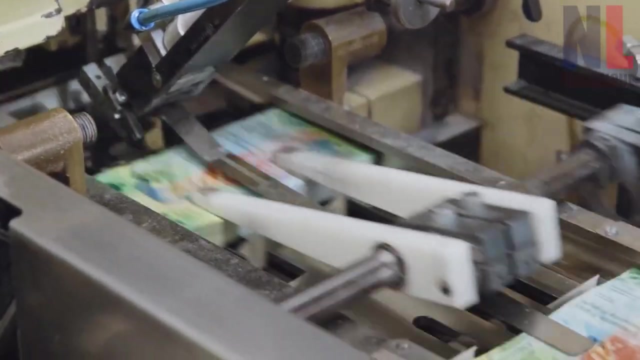 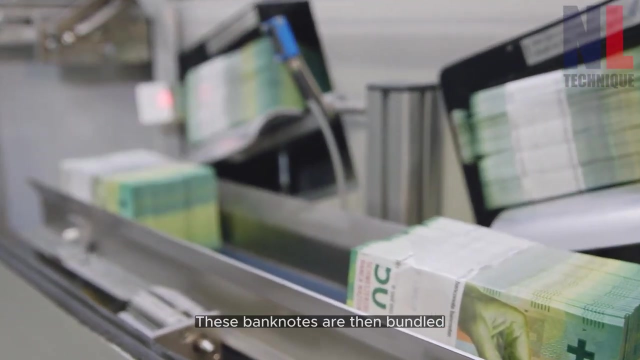 attention to detail guarantees that only the highest quality banknotes make it into circulation. finally, the banknotes are ready to be cut and packaged for distribution. specialized machines precisely cut the large printed sheets into individual banknotes. these banknotes are then bundled, sorted and prepared for distribution to banks. 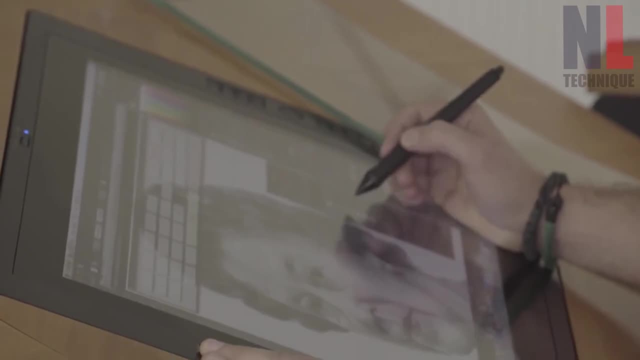 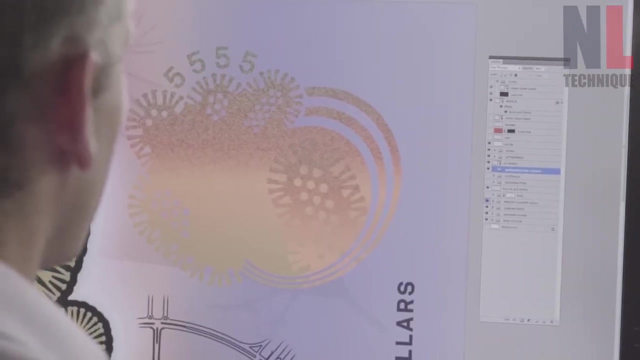 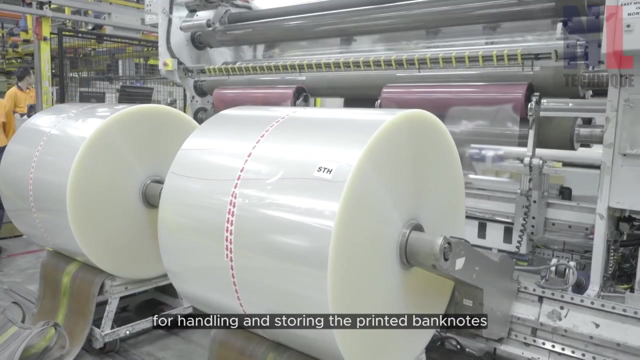 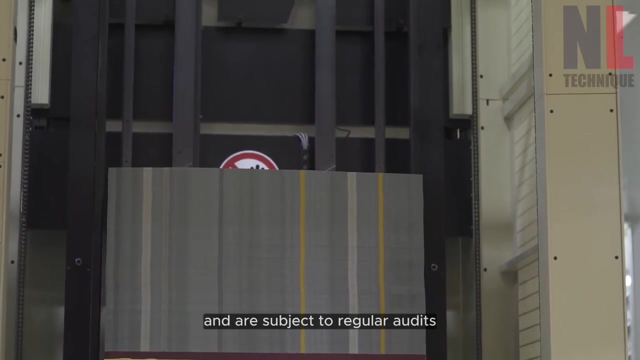 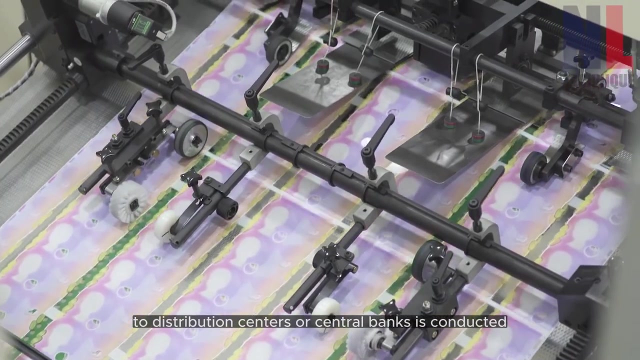 and financial institutions. the production facilities adhere to strict protocols for handling and storing the printed banknotes. secure storage areas are equipped with advance security systems and are subject to regular audits. transportation of banknotes from the printing facility to do the circulation efficiency, sleep distribution centers or central banks is conducted under strict security. 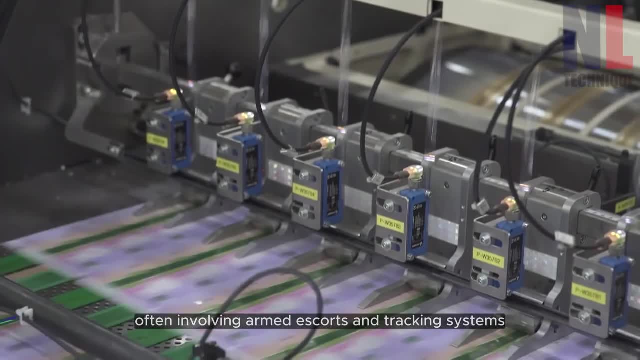 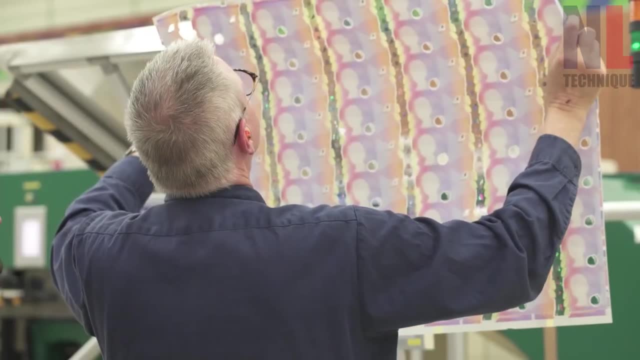 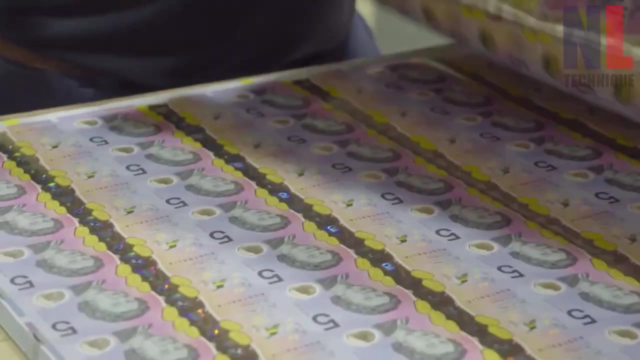 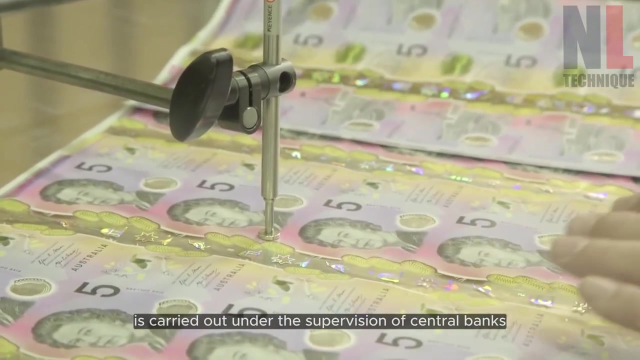 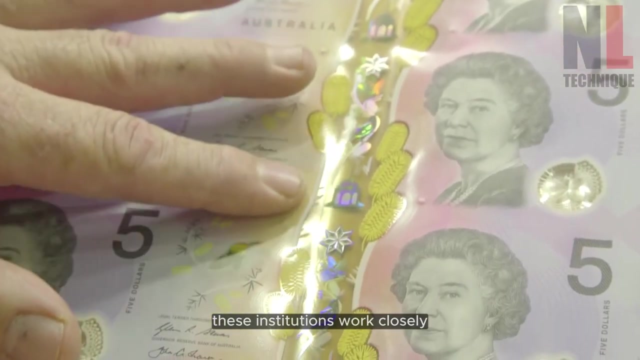 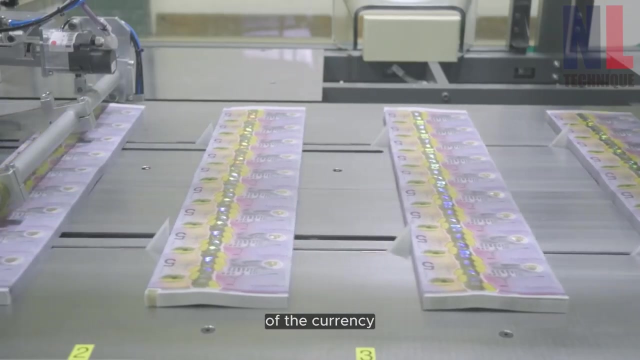 protocols, often involving armed escorts and tracking systems. furthermore, the printing process is carried out under the supervision of central banks or monetary authorities, which maintain strict oversight and control. these institutions work closely with law enforcement agencies and international organizations to combat counterfeiting and maintain the integrity of the currency. 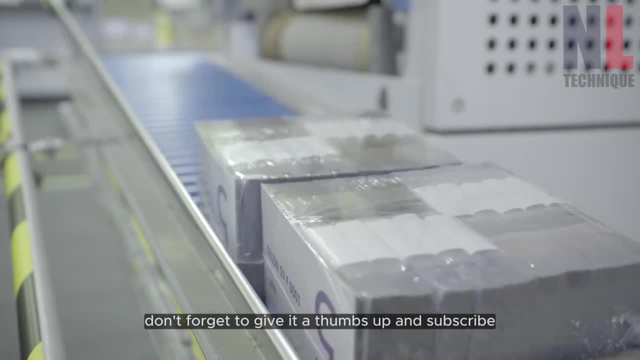 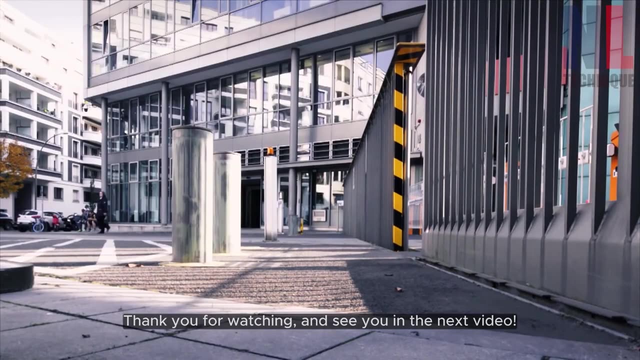 if you found this video informative, please like and subscribe to our channel. don't forget to give it a thumbs up and subscribe to our channel for more fascinating content. thank you for watching and see you in the next video.